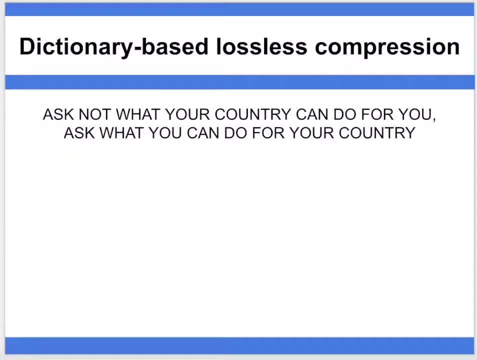 So dictionary-based compression is a concept which requires us to take the text and perform or create a dictionary of the words used in the text and then simply repeat them when they appear in our dictionary. So if we build an example up, Let's take this famous, famous quote, I believe, from John F Kennedy. 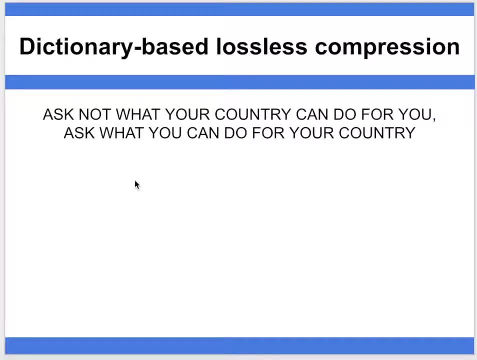 Ask not what your country can do for you, ask what you can do for your country. Now we can see that in a sentence like this, we actually have a series of repeated words that we can use to reference again and again. So what we would do in a dictionary-based compression example: we would create a new list. 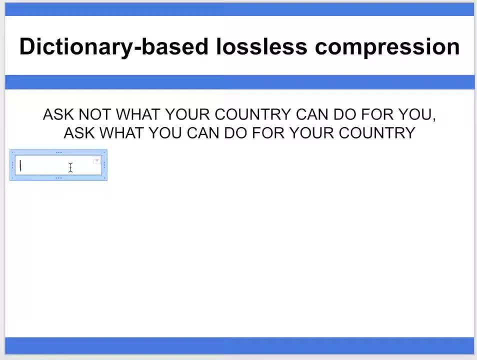 and we would interpolate it with all of the words that are uniquely represented within the actual sentence itself. So the word ask is the first word that we encounter and therefore is a unique word, Not what your country can do for you, And then we hit apply. 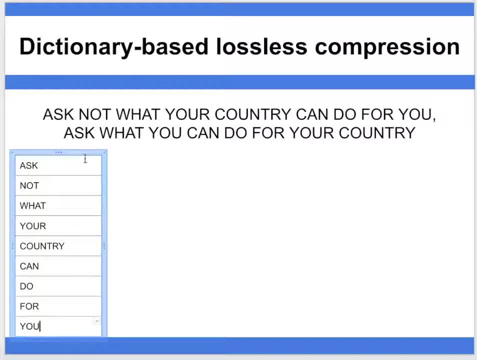 And this is the point where we have a repeat. So we have ask: is repeated twice now, so we don't put this in again. What is repeated already? You, we already have that. Can we have that? Do we've got that? 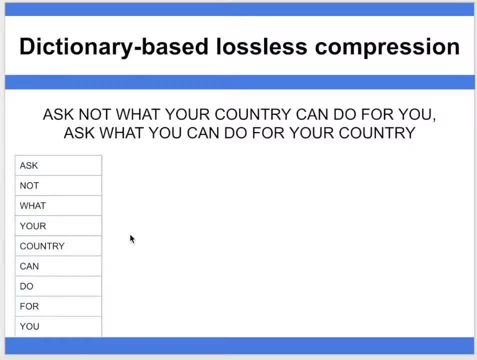 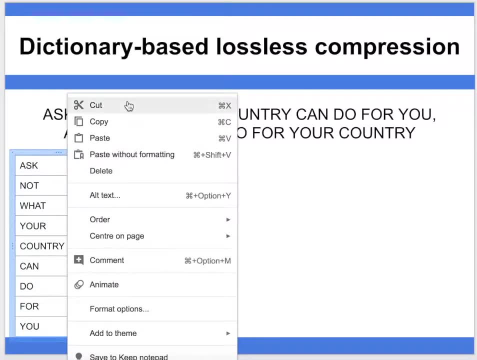 For got that again, Your got that, And then country. So, because this is now a list, and if we were programming this we would index from zero, and if we just put those indexes in just for the purpose of this, let's just add a. oh, hang on a second. 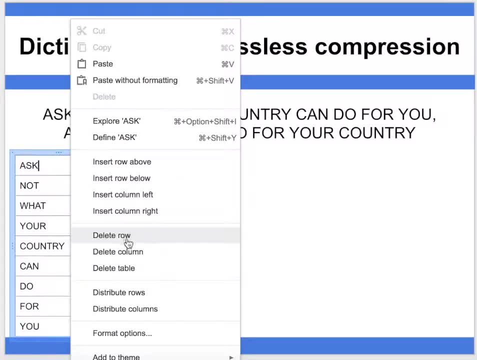 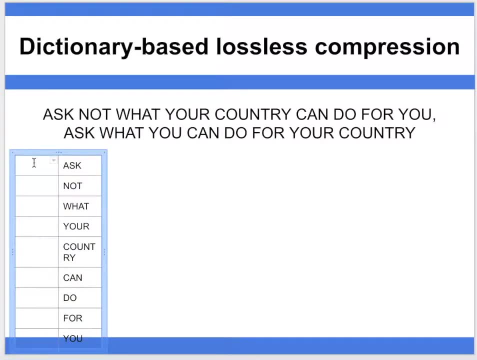 A bit crazy there. Let's add a new column in Column to the right, Column to the left, rather, And if we position these start with an index of zero, we have nine unique values in our list. So when we want to actually output this sentence,